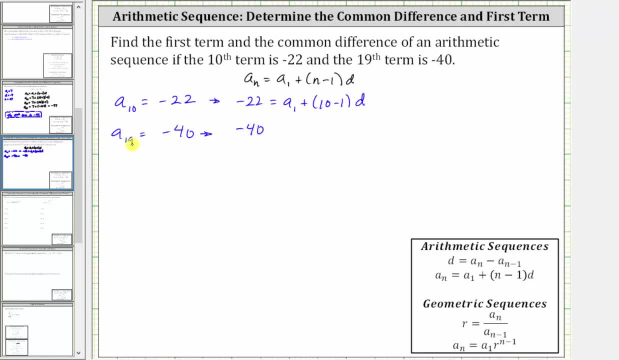 If we substitute negative 40 for a sub n, then we know n is 19,. giving us the equation: negative 40 equals a sub one plus the quantity 19 minus one times d. Simplifying here, we have negative 22 equals a sub one plus 90.. 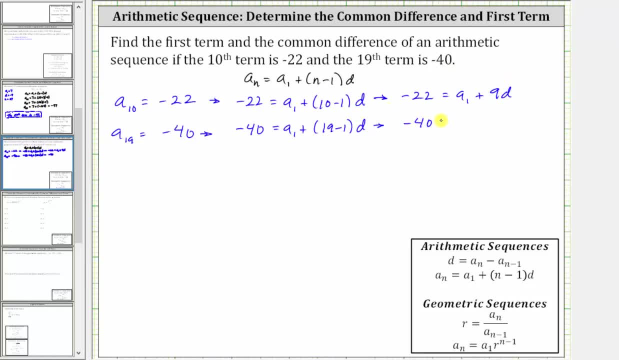 And the second equation. we have negative 40 equals a sub one plus 18d, And now we can solve this as a system of equations to determine a sub one and the common difference d If we use the method of elimination. notice how we have a sub one in both equations. 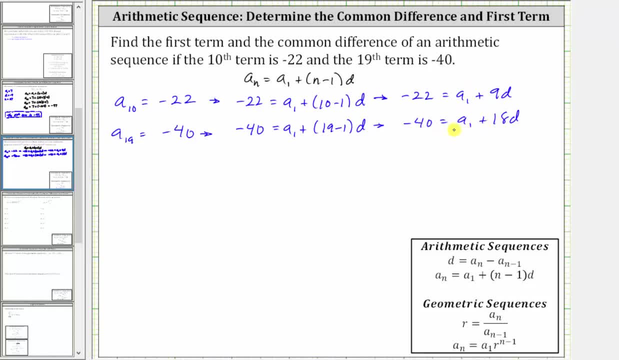 so we can subtract the two equations or multiply one equation by negative one and then add the equations. So let's rewrite the equations down here: We have negative 22 equals a sub one plus 90, and we have negative 40 equals a sub one plus 18d. 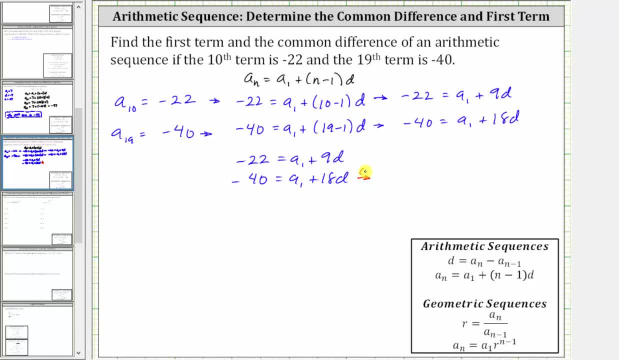 Let's multiply the second equation by negative one, leave the first equation the same, and then we'll add the two equations together, So the first equation stays the same. Now we multiply both sides of the second equation by negative one, which gives us positive 40. 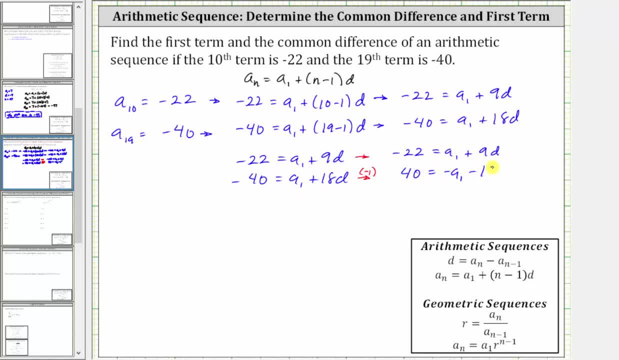 equals negative, a sub one minus 18d. And now we'll add the two equations together: Negative: 22 plus 40 is positive, 18 equals a sub one plus negative, a sub one is zero. So these terms simplify out: 90 plus negative, 18d is negative, 90.. 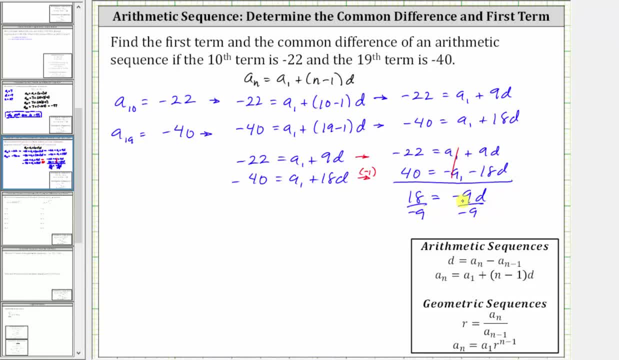 So now we divide both sides by negative nine and simplify, and we have: d is equal to negative two. So now that we know d is equal to negative two, we know the common difference is negative two. And now to determine a sub one. 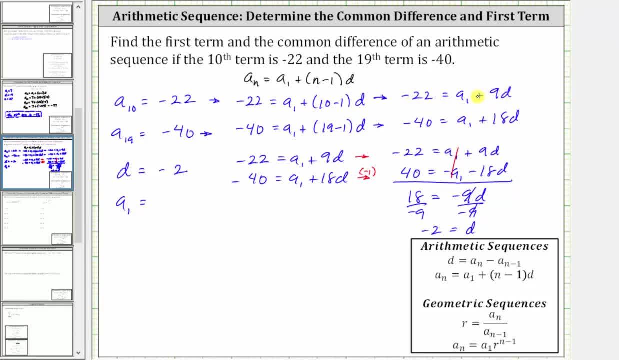 we can use either of the equations that we formed. Let's use this equation here, Where we know that negative 22 equals a sub one plus nine d. So now we can substitute negative two for d and solve for a sub one, giving us negative 22 equals a sub one.